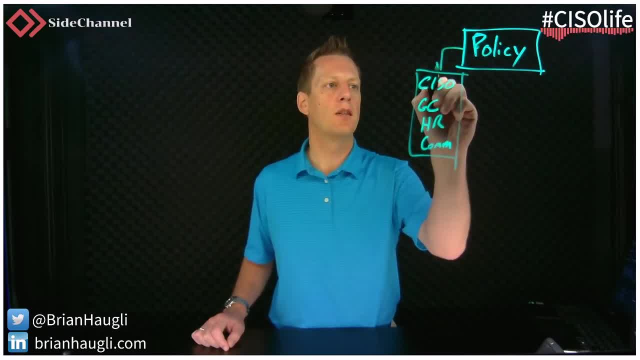 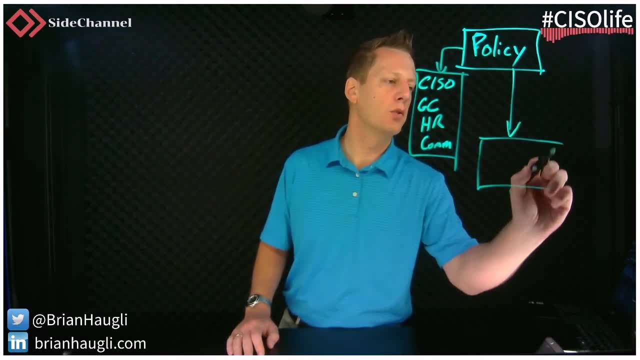 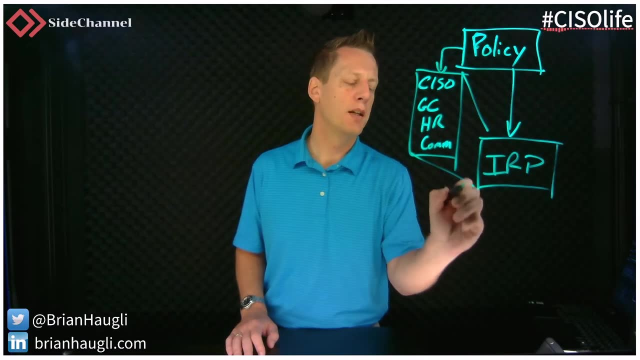 OK, You need to create the power for this team to be able to actually go do its job. And what's that policy going to do? It's going to allow you to craft an incident response Plan, And this is exactly what this group is going to work on and use and hopefully read before you actually need to go do it. 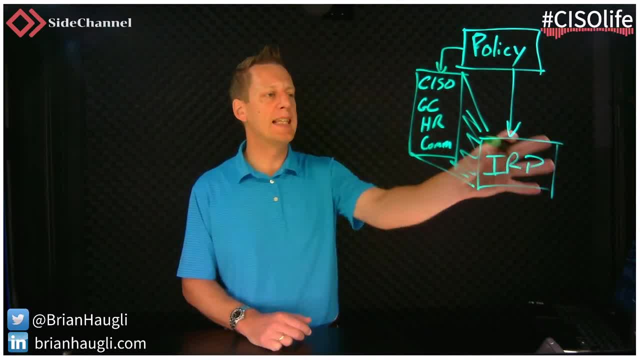 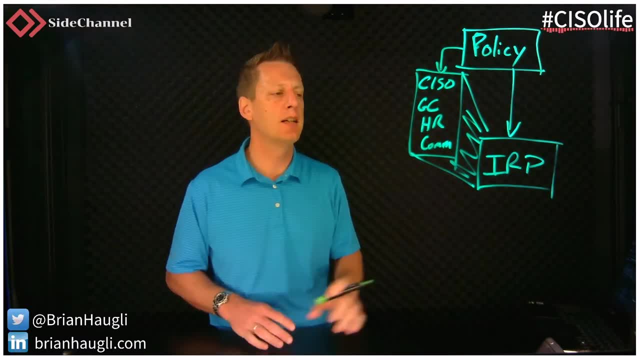 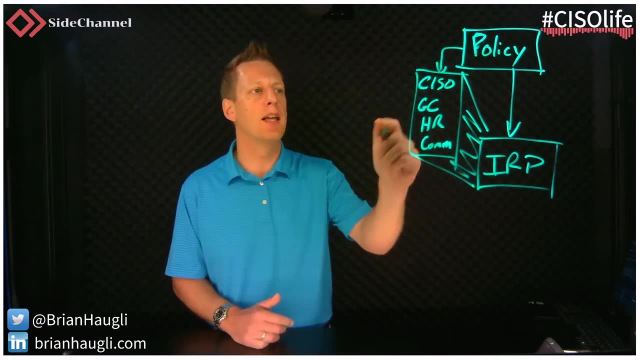 This IRP, an incident response plan. This is what you follow. So your policy empowers the team, empowers the ability that the IRP, as you're going to build it, is going to have the power and the authority to go do what is needed by this team and their group. 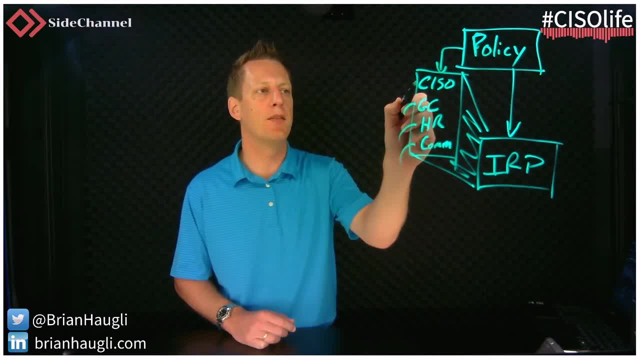 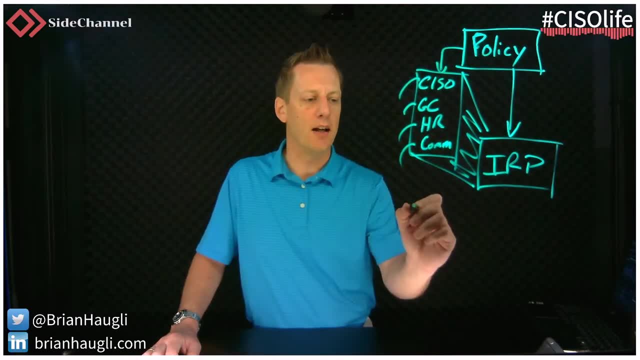 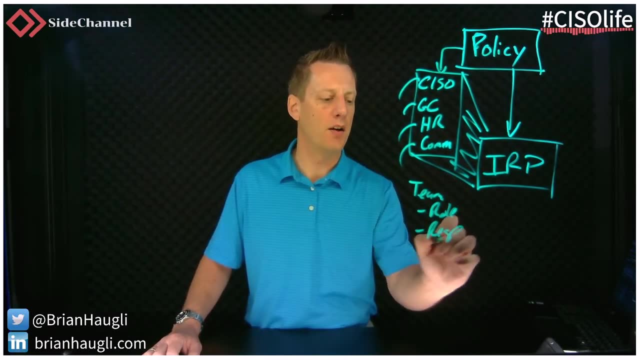 So you're going to have a legal team under GC and HR team, A comms team and, obviously, an infosec team underneath your CISO. So what does an IRP end up looking like? Well, it's going to again. it's going to outline who the team is, OK, what their roles are, what their responsibilities are. 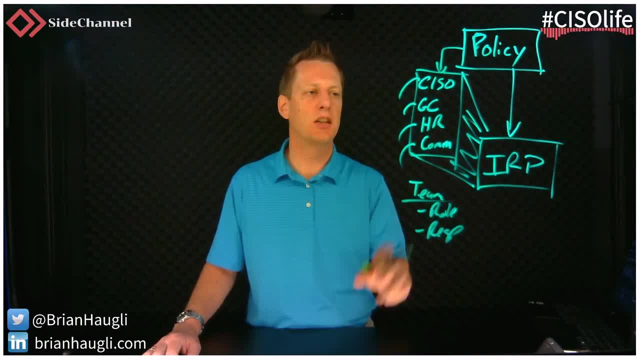 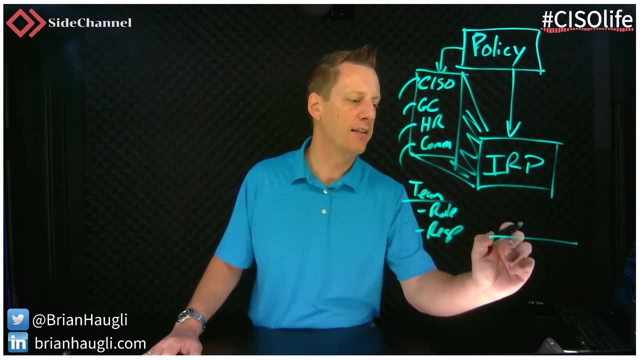 OK. this is very important. You need to clearly define inside of an incident and its response. You need to define who has what role. Do you have an incident commander? Do you have a group that has the authority? Do you have the authority to discuss when the incident right? we're now left of boom, OK, or we're now right of boom, sorry. 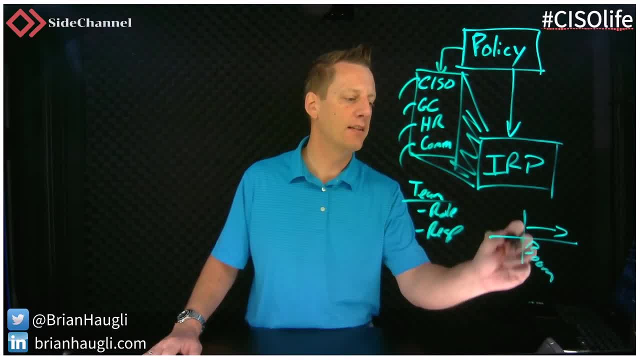 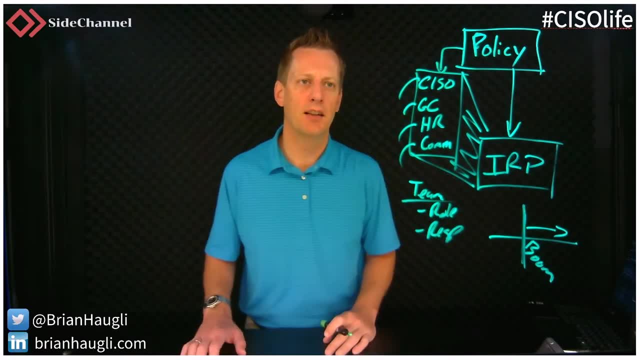 What? when do we say that this is a breach? OK, who makes that call? OK, that needs to be outlined. OK, you need to have some type of a matrix. There's a lot that goes into this, And it's a great area that we like to work with clients. 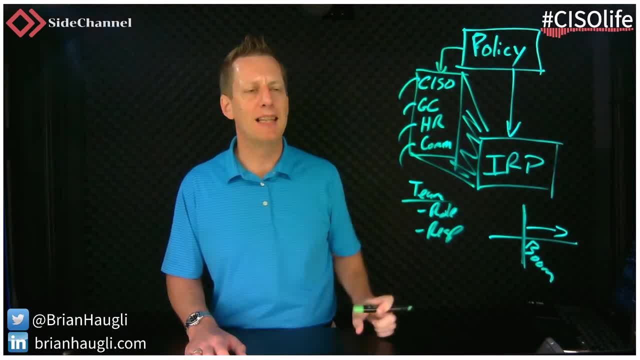 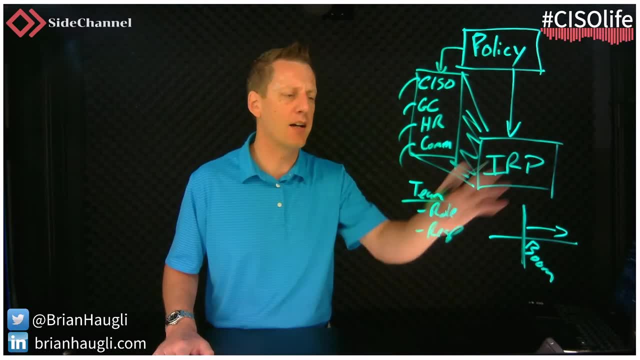 We fly in some accelerator documents and we build these out based on who you have, What you have available, what resources, the culture, the thinking, what are you trying to protect? OK, not every IRP is going to be built the exact same. 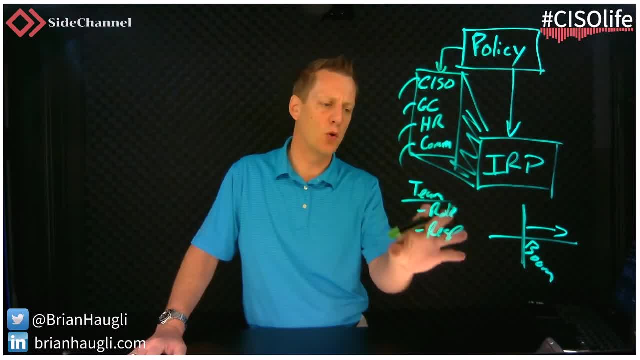 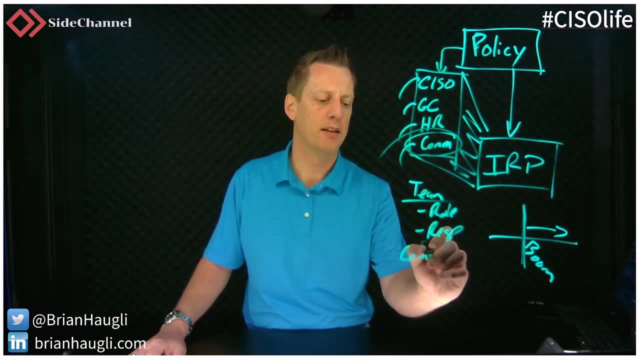 So you want to be able to have your team, the roles, the responsibilities. OK, you want to really key in on your communications group? OK, what does the comms look like? OK, this is super important. When do you make that call? 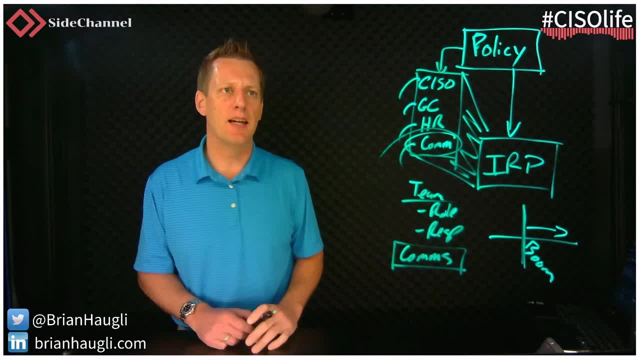 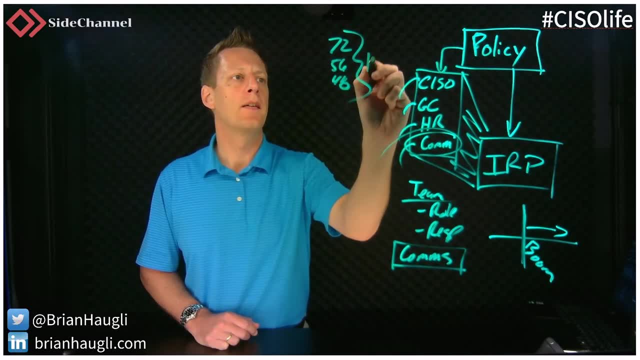 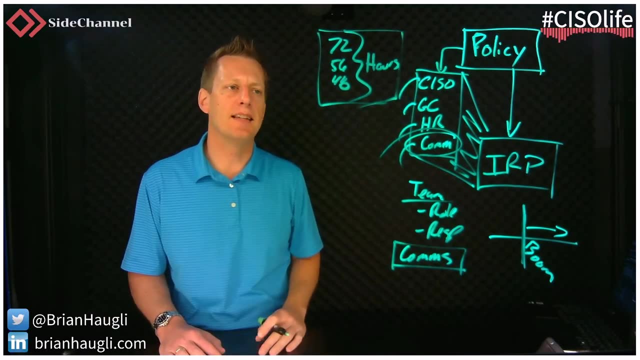 OK, do you have a regulation? that's sitting out there that's saying, hey, you know, within 72 hours, 56,, 48 hours, OK, you need to be notifying someone. Is it a regulator? Is it the SEC? 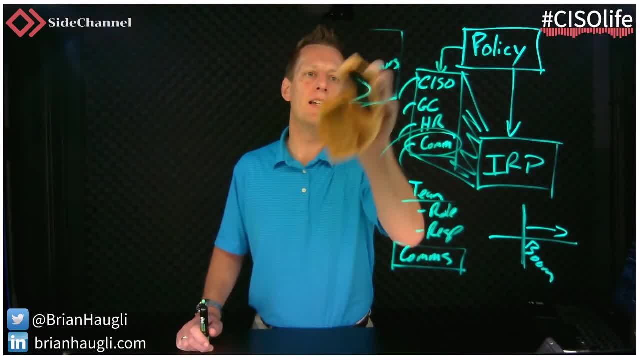 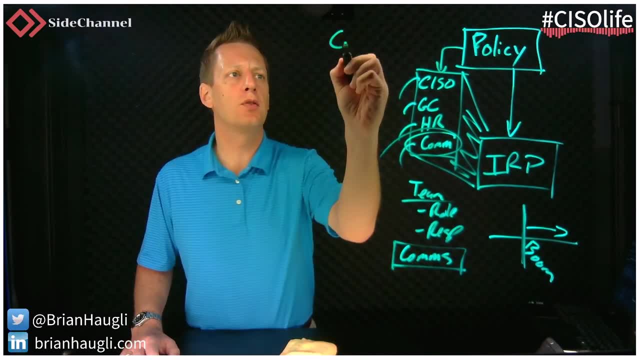 Who is it? OK, you need to be able to have that nailed down. If you don't have that internally, when do you want to be speaking to your customers? OK, Your shareholders, right? Maybe the SEC, because you're publicly traded. 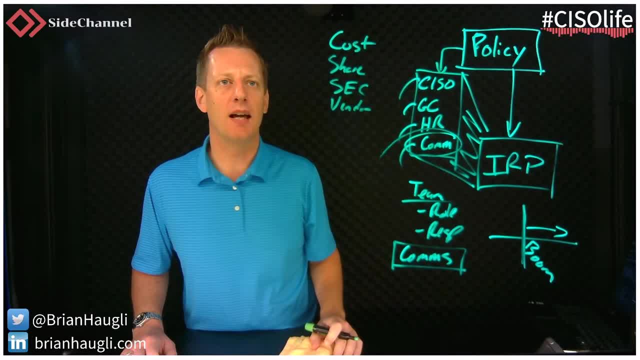 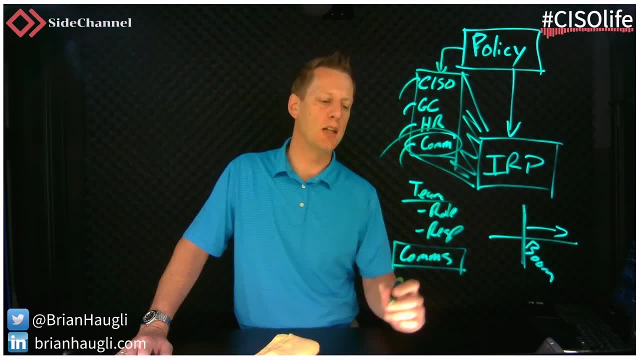 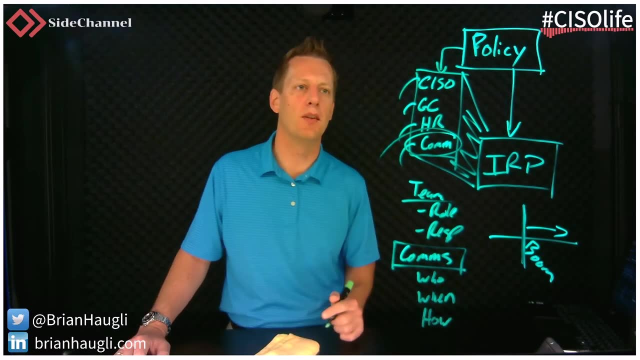 OK, maybe it's a key vendor. OK, that's, you know, an upstream or downstream problem for you. You need to determine where your communication is going to hit, when you need to do that communication. OK, so you got to address who, when and, obviously, how are you communicating with them? 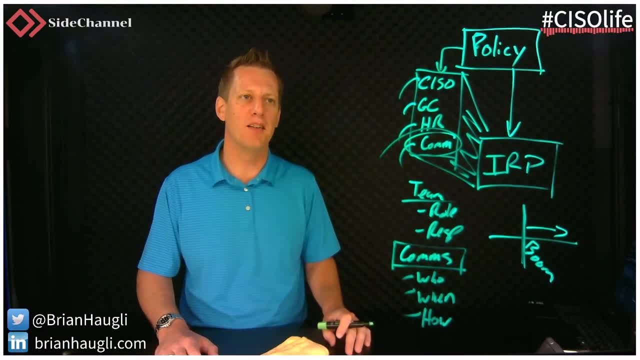 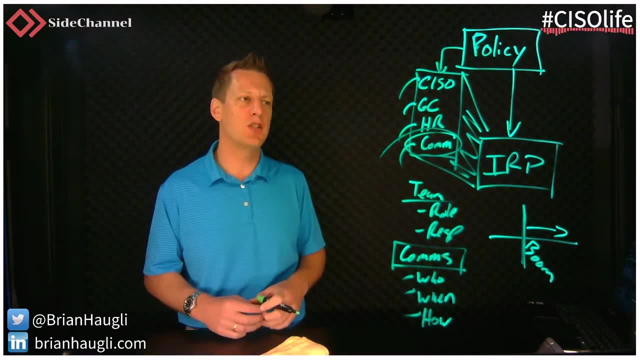 You know the default is: oh, we'll email them. Well, what if your email system is compromised? Do you want to let on? Do you want to let on to the attacker that you know that they're in there, that you're breached, that you're orchestrating a response? 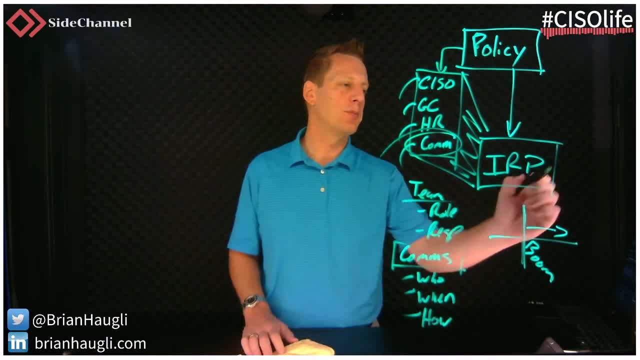 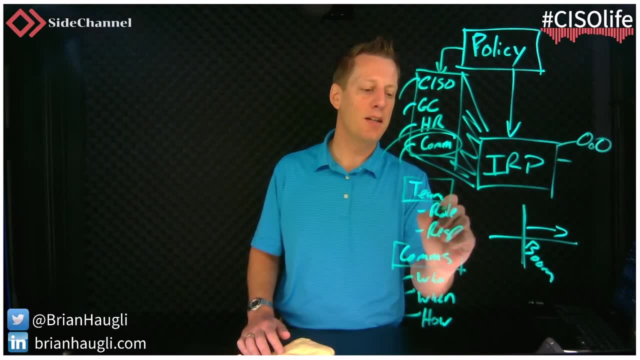 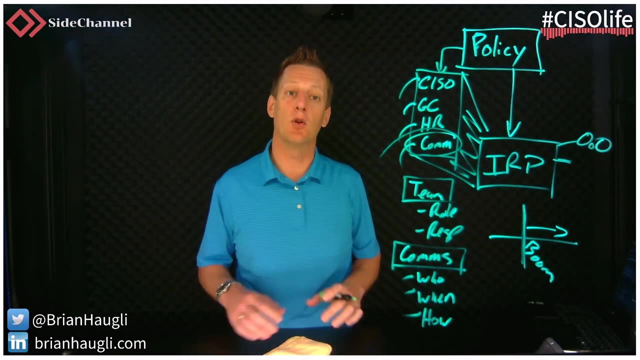 Probably not. So you know, this plan has to have some type of out-of-band comms. It needs to have quite a bit OK, and it's really interesting, as you start building this out, what you learn about a client or your own company as what's needed and what's missing. 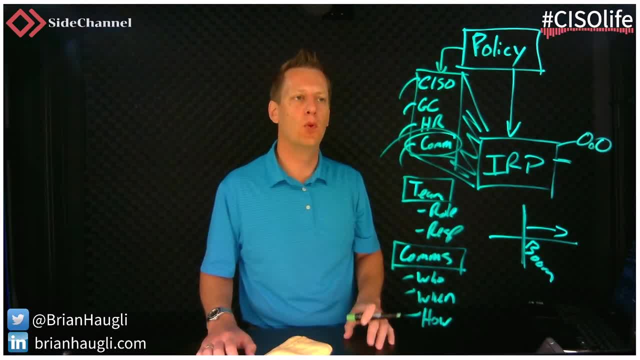 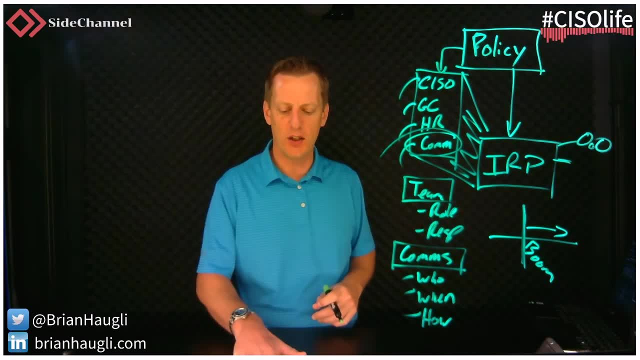 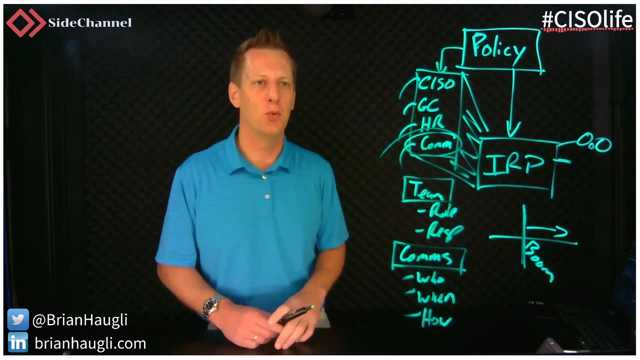 And going through this process Here really helps you define your team. your cybersecurity capabilities really hone in on gaps that exist within this. A lot of people walk into this thinking, oh, we've got this in place, this is already all set, we're good. 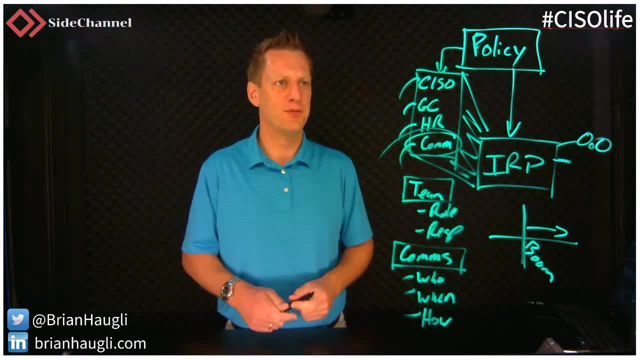 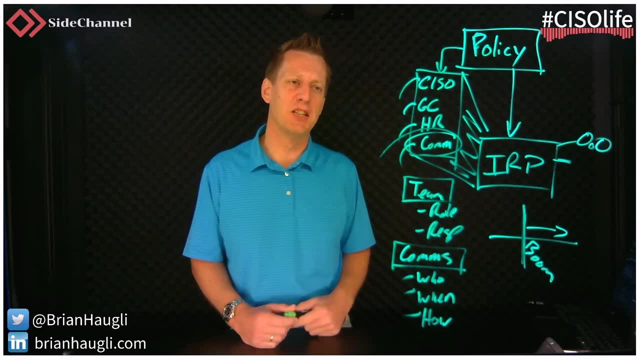 And then you start actually unearthing. hey, has anybody ever read this? If you do a tabletop, is half the tabletop team opening this for the first time. That's not going to be a good day if you have, if all of a sudden you write a boom. 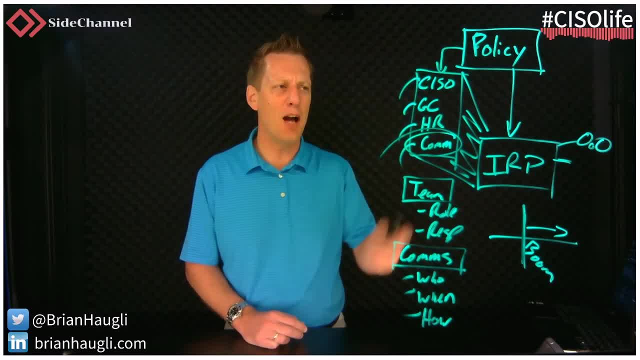 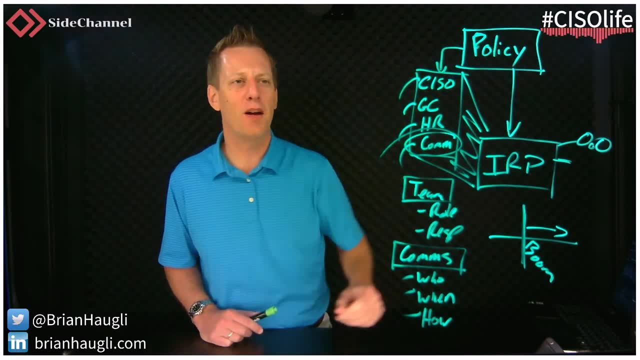 All right, folks. anyway, some great areas to key in on. How many of you are doing this right? Comment down below. Let me know how many have a policy that empowers a team, has an incident response plan that clearly articulates these things, and a host of other areas that you've got to get into.